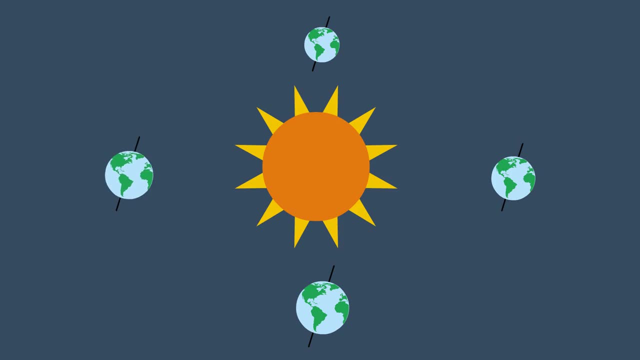 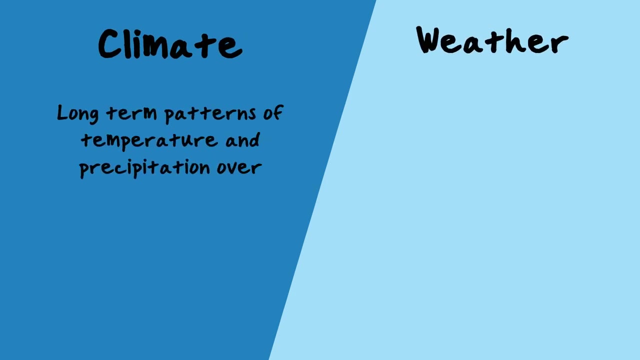 is farther away from the Sun, giving it colder climate. Now it's important to make a distinction between climate and weather. Climate is the combined long-term effects of temperature and precipitation patterns. It's climate that determines the type of environmental conditions in an area like whether it's a desert or grassland. The climate that determines the type of environmental conditions in 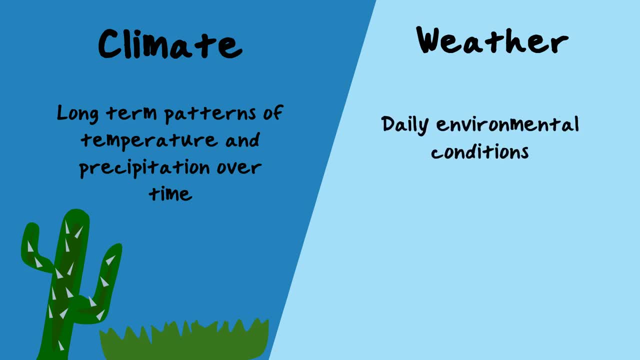 an area like whether it's a desert or grassland. The climate that determines the type of environmental Weather is short-term conditions in a particular area, whether it's sunny or cloudy or rainy, While weather can be used to determine things like what outfit to wear on a certain day. 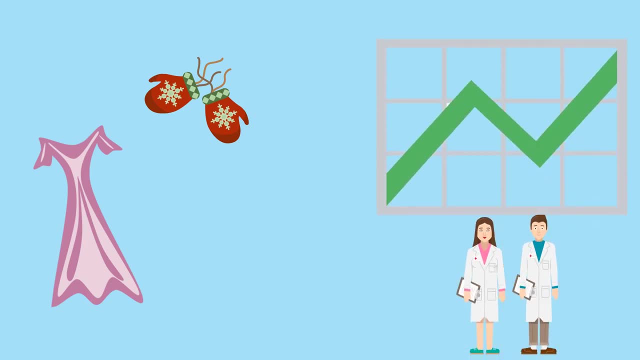 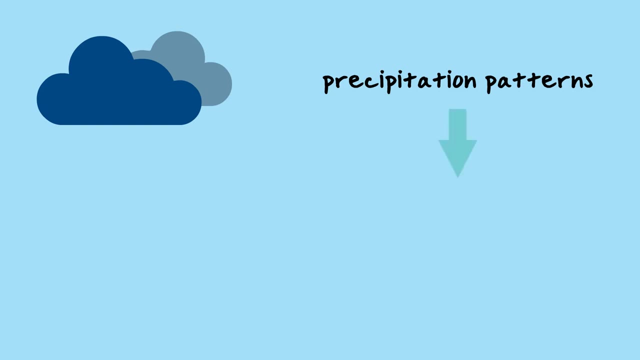 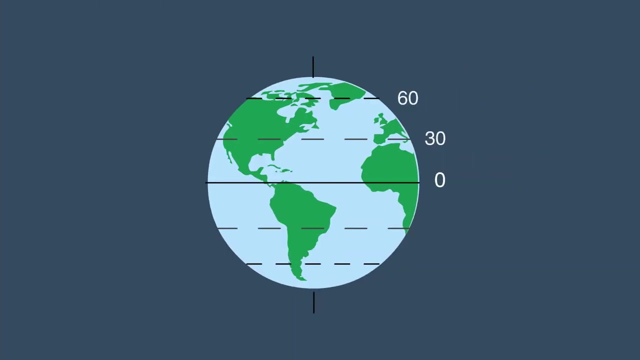 long-term pattern, or climate, is what scientists study to measure climate change. Also, the amount of rainfall in an area determines its climate, which contributes to the type of vegetation that will grow there and, consequently, the biome. Now that we have an understanding of the difference between weather and climate, 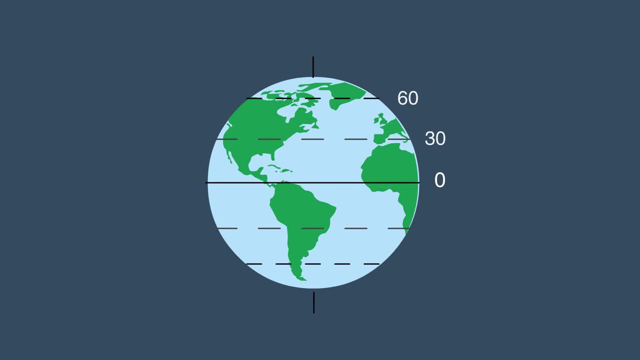 let's talk about precipitation and wind currents a little bit more and how their patterns vary across the planet. If we look at our planet, we see constant cycles of rising and falling air, which are created as a result of precipitation and temperature patterns in different latitudes. 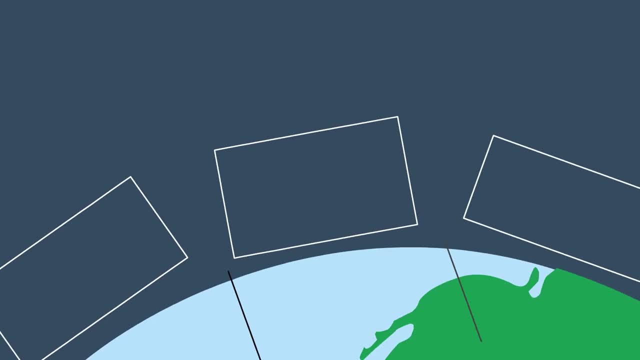 Let's start with the Hadley cell, which starts around 0 degrees and goes until 30 degrees At the equator. the heat causes hot, humid air to rise. The evaporated water in the air falls back down as rain. 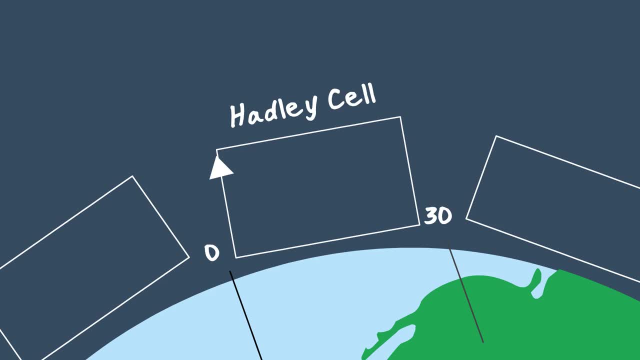 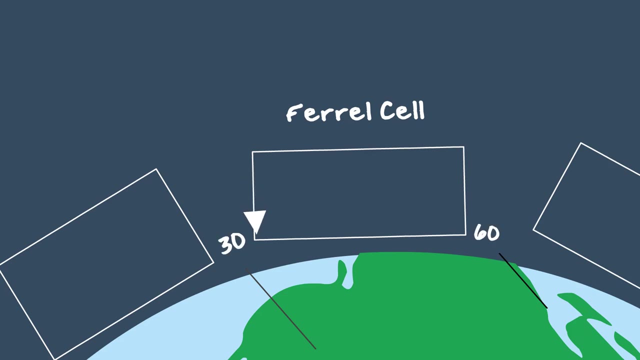 making the air really dry. This hot, dry air then moves, cools and falls back down at 30 degrees. The next cell, called the ferrule cell, has cooled dry air, falling down at 30 degrees, which then sweep across the Earth and warm up. 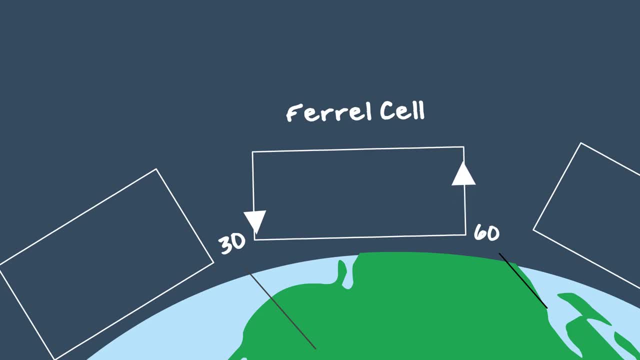 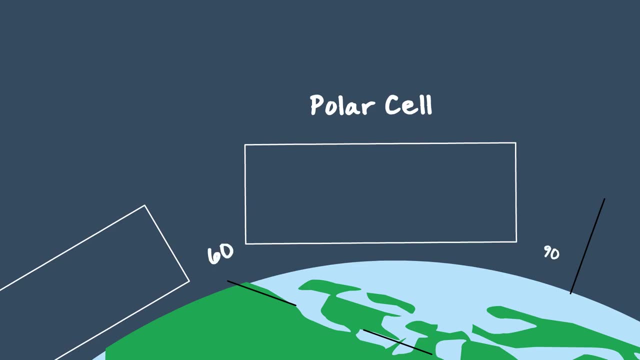 As it warms again, it rises around 60 degrees. The final cell, Called the polar cell, has warmer air, rising at 60 degrees. Similar to the Hadley cell, it starts to cool down as it travels sideways before finally falling back down at the poles.